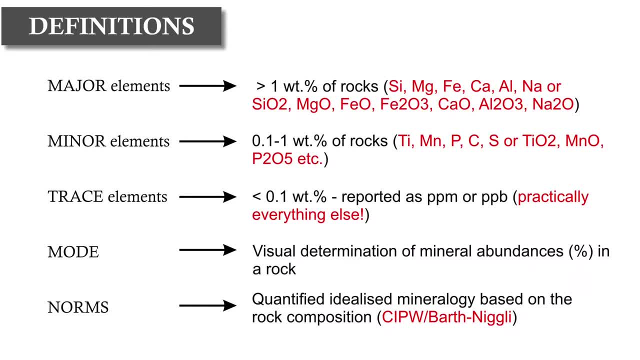 And then we have minor elements, and minor elements comprise between 0.1 to 1 weight percent of rocks, so they're still key components, but not as essential as the rock forming elements, and these include things like titanium, manganese and phosphorus. Each of these are also most. 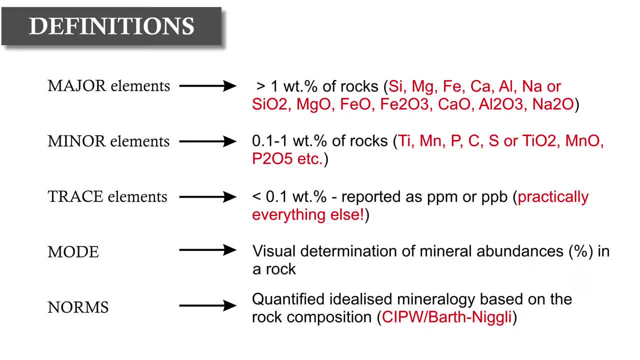 commonly referred to as rock forming elements. So these are the elements that are most commonly represented in geochemistry, and these are also the most commonly represented in geochemistry, reported as oxides, but then also things like carbon and sulfur, depending on the rocks that we're working with, And then, finally, we have the trace elements, and this is essentially a group. 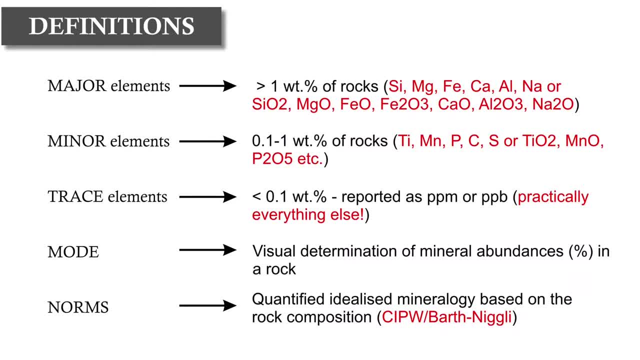 term for everything else, and these are elements that have concentrations below 0.1 weight percent and because of this they're most often reported as parts per million or ppm, or parts per billion or ppb, And I have a couple more definitions here. so mode: mode represents the visual determination of 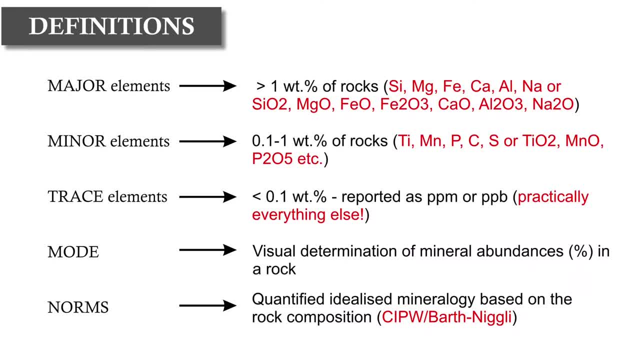 mineral abundances in a rock, typically reported in percent. So, for example, say that we're looking at a gabbro that has, you know, half of its mineral component is plagioclase. that rock would have a 50% mode of plagioclase. And then, below that, we have norms or normative calculations and these 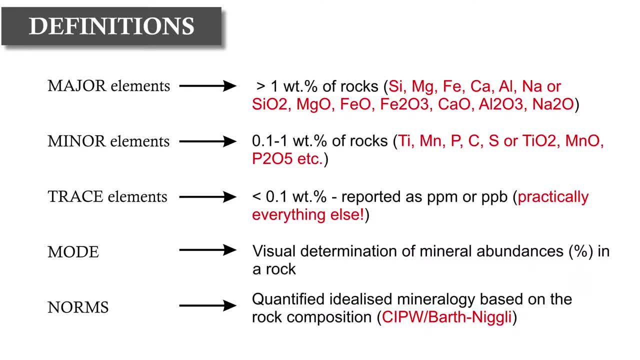 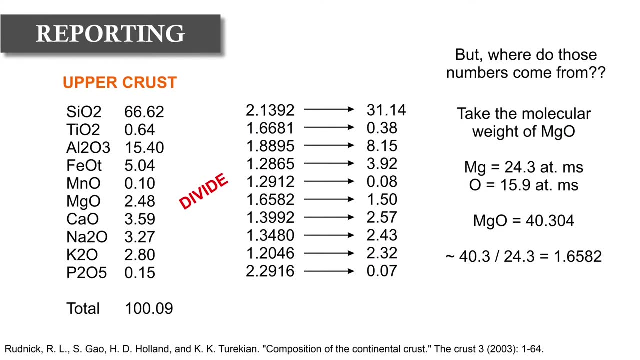 are quantified, idealized mineralogies based on the input composition of a rock. So we take the oxide composition of our rock, we perform some calculations- common examples are CIPW or Barth-Nigley method- and this produces a mineralogy for the rock. So when we report, 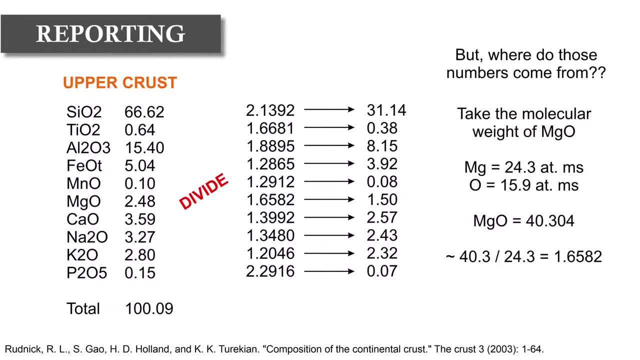 geochemistry, we typically report it as weight percent oxides, in the order that I have to the left of the slide, and what we hope is that these oxides will generally add up to equal around 100 weight percent. Now, this isn't always the case, due to things such as analytical uncertainty and also 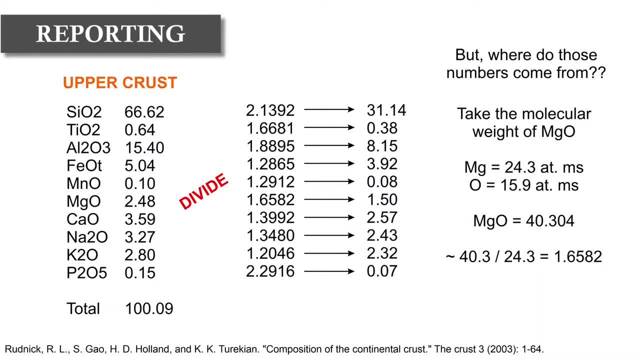 things like detection limits and we're kind of looking between a range of 99 to 101 weight percent on the method that we're using. of course, Now the major elements, the rock forming elements, are typically reported as oxides in this case, but if we did want to report it as individual elements, 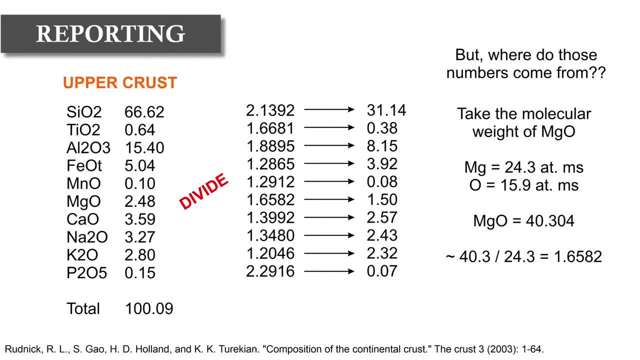 ie we want the silica weight percent rather than the silica dioxide weight percent. we can perform a fairly simple calculation to convert between the two. So what we would do is we would take these conversion factors I've reported in the middle, which are freely available online. we would take 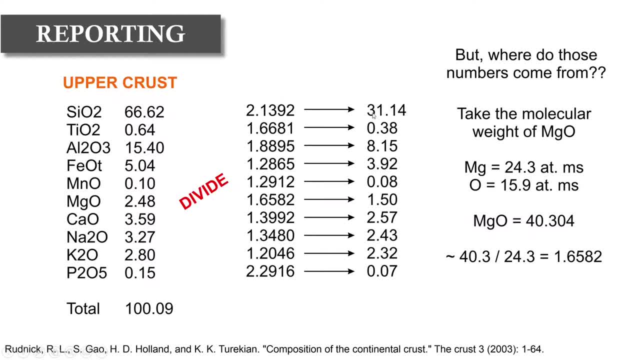 our weight percent oxide. divide it by the conversion factor and we would get our weight percent of magnesium oxide. This is a very simple example, but it's good to give a bit of background of where these numbers actually come from. So I'll give an example here for magnesium. So if we take the molecular weight of magnesium, that is, the atomic mass units of magnesium and oxygen added together. as we have one ion of magnesium, one ion of oxygen, this is just one each, and so the molecular weight of magnesium oxide will become 40.304.. We would take our molecular weight of magnesium oxide, divide it by the. 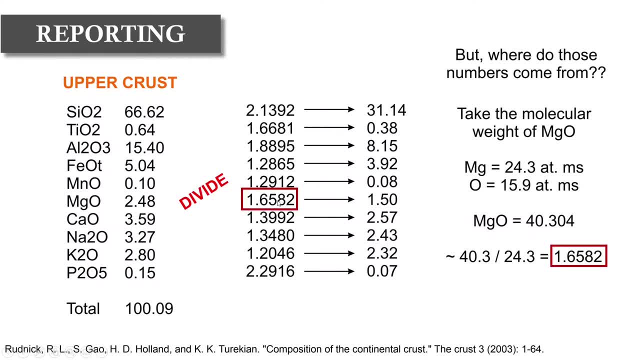 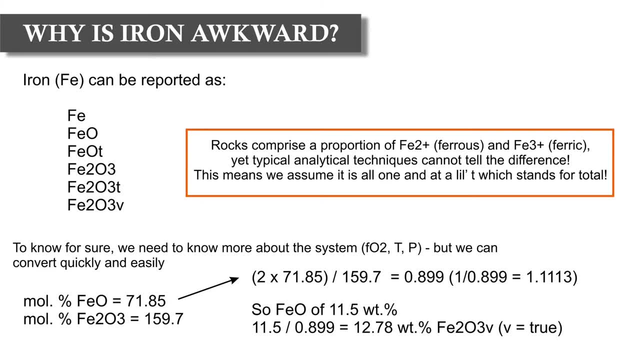 atomic mass units of magnesium, we would generate 1.656.. 2582, which is the conversion factor that we're using Now. iron can be quite tricky because it can be reported in a number of ways. so it can be reported, obviously, just as iron it can be reported. 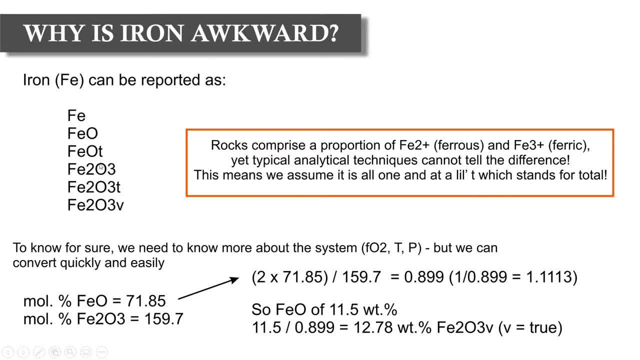 as ferrous iron and it can be reported as ferric iron, and it can also be reported as both, with a small t on the end, and that t stands for total. The reason it can be reported in a number of ways is because rocks comprise a variable proportion of ferrous and ferric iron, and typical analytical 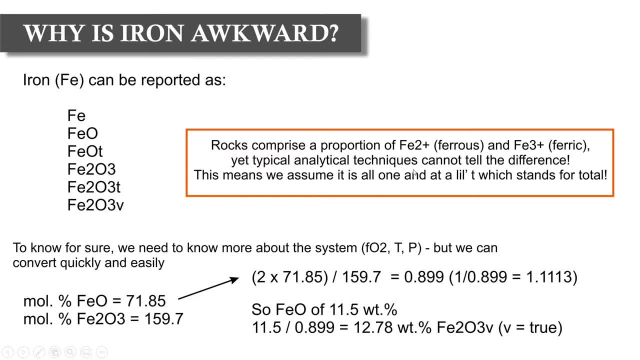 techniques that we use can't tell the difference between these two types of iron. So what that means is that when we analyze the rocks, the machines assume that all of the iron it's measured is one or the other. so that's where that t comes from. it's saying: okay, we've measured the iron in. 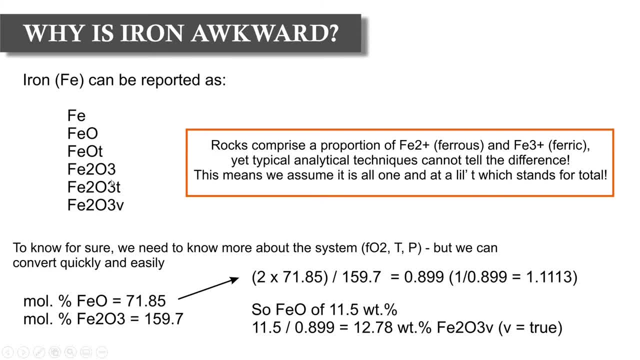 the rock and we're assuming it's all ferrous iron or ferric iron. so that's where we get the small t. If we wanted to know the exact proportions of how much ferrous and how much ferric iron were in the rock that we're analyzing, we'd need to know a little bit more about the system, about the conditions. 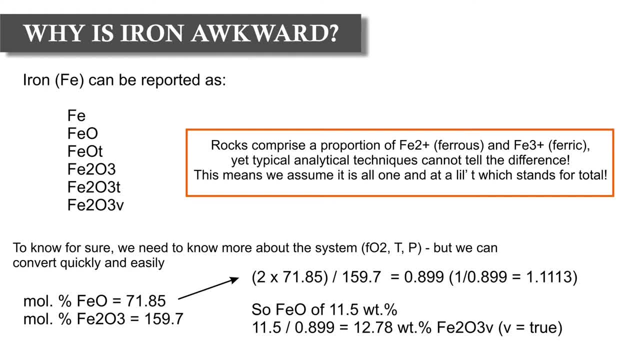 that rock crystallized under. This includes things like oxidation state, temperature, pressure, so this is really more important for academic purposes. We can perform quite a rudimentary calculation to convert our weight percent between the two ferrous and ferric oxide, and I've given a. 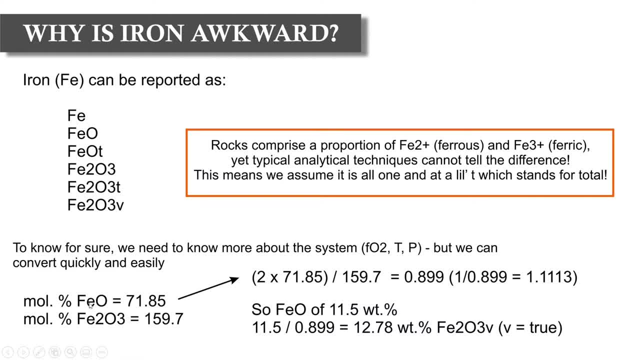 small example here. What we would need to do is we would need to calculate the molecular weight of both of our ferrous and ferric iron, just as we did for magnesium oxide in the previous slide. We would multiply our ferrous iron molecular weight by two, purely because ferric iron has two. 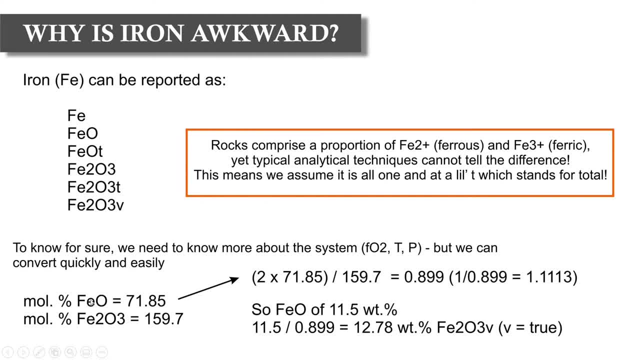 ions in its formula, whereas ferric iron only ferrous iron only has one. and then we generate this, this formula here, where we have two times ferrous iron divided by the molecular weight of ferric iron, and it gives us a conversion factor of 0.899, which is sometimes also reported as 1.1113. 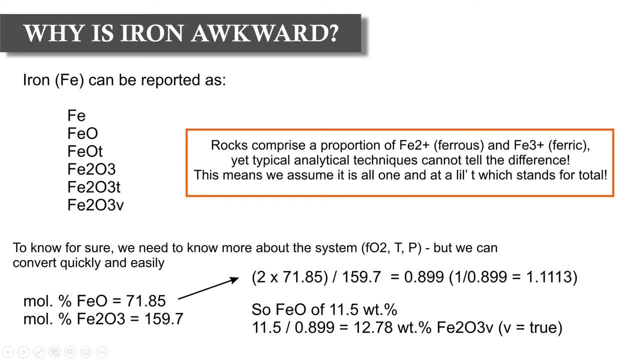 which is essentially just one over our conversion factor here. So therefore, if we have a 11.5 weight percent of ferrous iron, we would do 11.5 divided by our conversion factor, we would generate a weight percent of ferric iron of 12.78 weight percent, and sometimes we might. 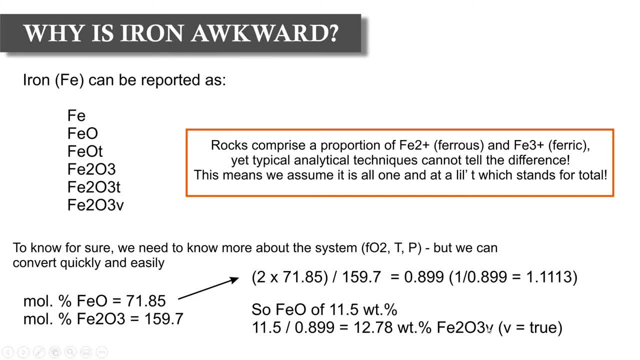 proceed that by a small v, which is in French for true, so fray, and that essentially tells us that this is recalculated iron. Now, this can be quite important. if you're compiling data from different studies that report iron in different ways, it's important to know that you know these, these. 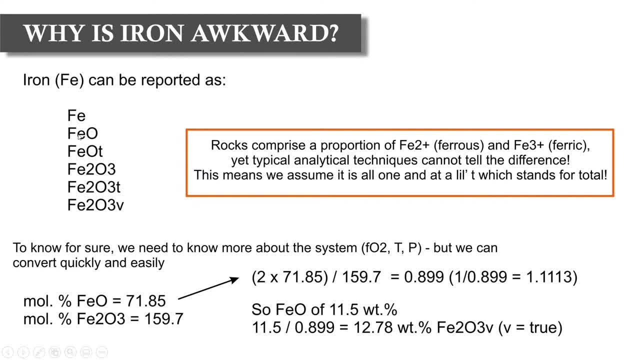 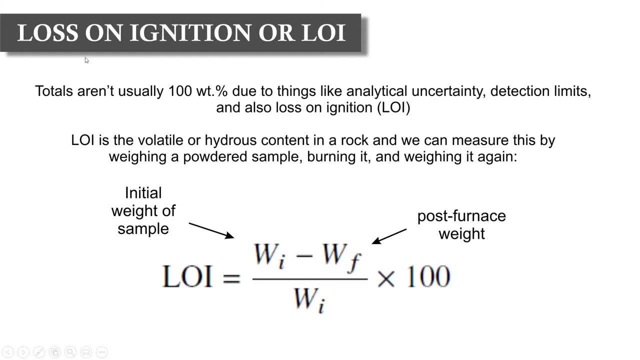 different ways that iron reported are not interchangeable and we would have to counteract that if we are doing some sort of compilation Loss on ignition or LOI. So loss on ignition is essentially the volatile or hydrous content in a rock. that's sort of locked away within hydrous minerals, and this is another reason as to why. 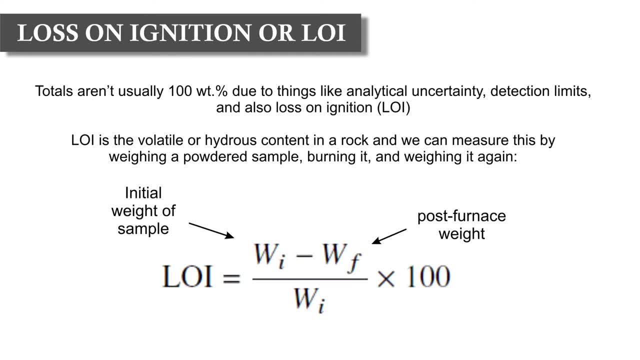 the totals of our weight percent oxides might not be 100 percent. How we would measure loss on ignition is we would take our powdered rock sample, we would weigh it, we would put it in a furnace and burn it for a short while and then we would weigh it again. and during the process of 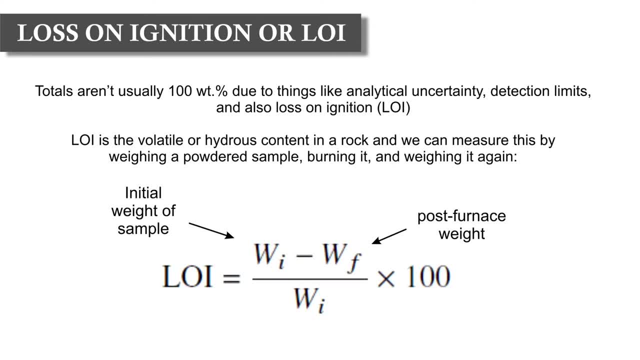 burning, a lot of the water and volatile content has been burnt off and it is through the difference of weight in our before and after that we can calculate the weight percent of LOI. So you can imagine if we have a relatively fresh basalt with not many 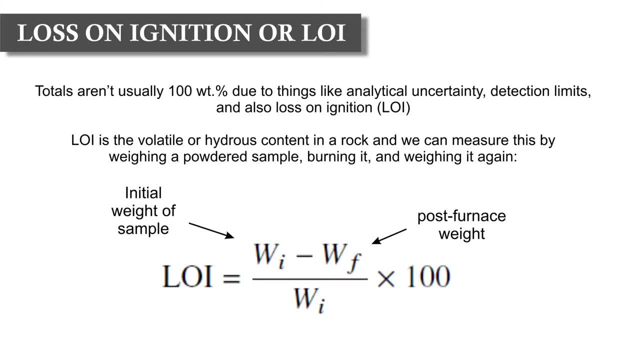 amphibole or mica phases, we would have quite a low LOI, whereas if we had quite a heavily altered rock- maybe it's been serpentinized- we would have quite a high LOI weight percent. So now getting some common diagrams, and perhaps one of the most common geochemical diagrams is: 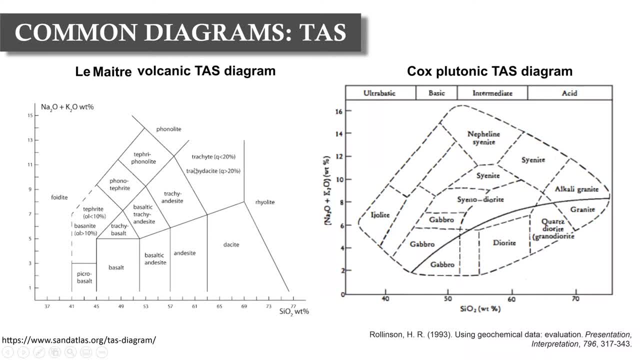 TAS, or total alkali silica. I have two examples here: I have an extrusive volcanic example and I have an intrusive plutonic example. So at the base we have silica dioxide and on the y-axis we have alkalis, which are sodium and potassium oxide phases, and in the middle we have geochemical 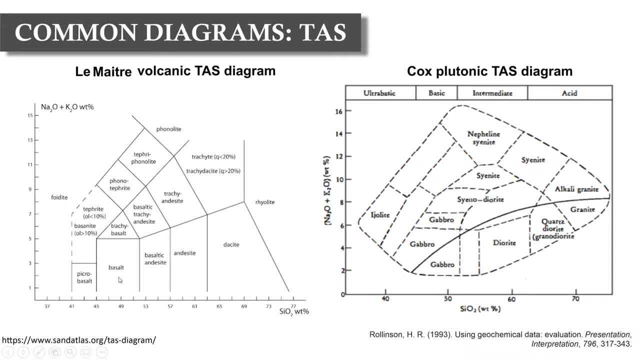 fields where the chemistry within them corresponds to that particular rock type. and there are probably some rock types that you recognize, ie basalts and things so on and so forth. Now these are obviously quite important tools for rock classification. but if I just plot some examples here, so if we take 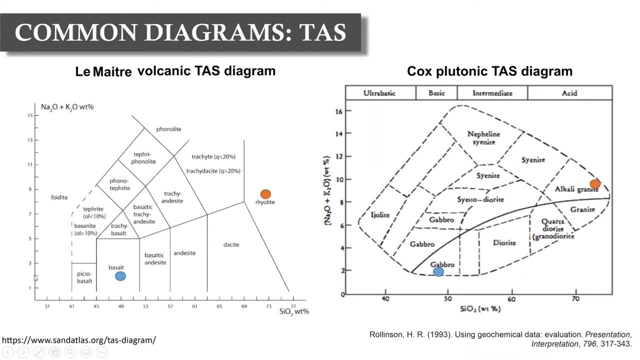 a geochemical which plots at around 49 weight percent silica and around two weight percent alkalis. the rock. this rock corresponds to a basalt, whereas if we use this classification, this rock would correspond to a gabbro, Gabbro being essentially an intrusive variation of a. 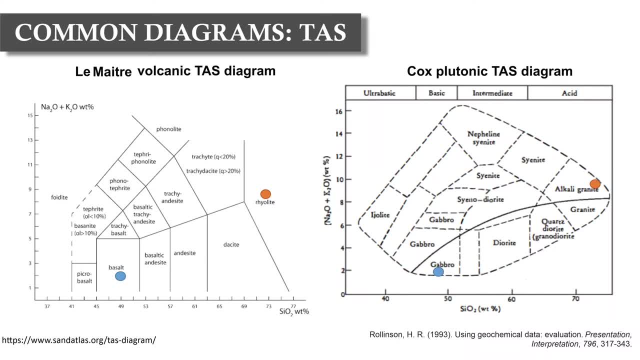 basaltic rock. So this is quite important- say we didn't know anything else about a rock and we just had the geochemistry. one might say that this is a gabbro or a basalt, when it could be one or the other. So this is an important lesson, for you know, the rocks always come first. 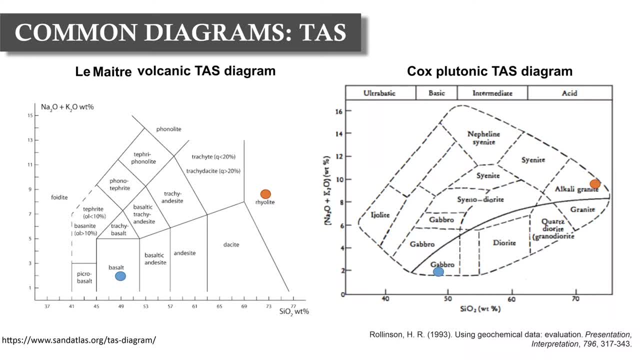 So we'd have to look at the rock to fully determine what this rock type is. you know, just geochemistry alone isn't important. Geology is all about rocks. and then we have our orange circle here, which is the same. so it can either correspond to a rhyolite if we're looking at a fine-grained. 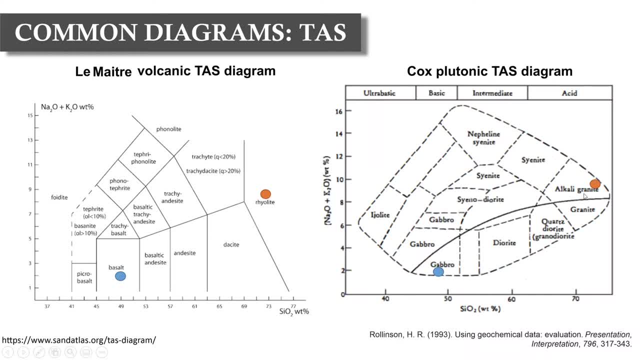 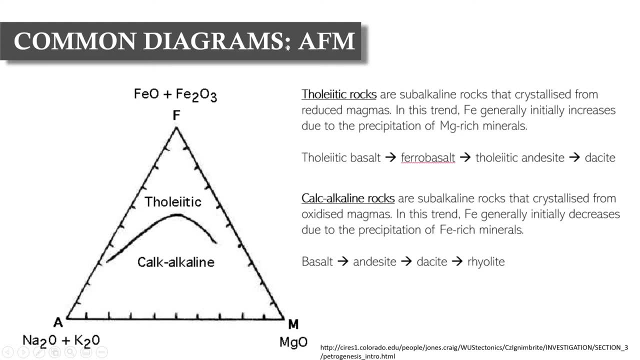 volcanic rock or some type of granite. if we're looking at a coarse-grained plutonic rock, Quite important. Another common diagram used in igneous rocks is what's referred to as the AFM diagram, which is presented as a ternary diagram. In the bottom left we have our alkalis. 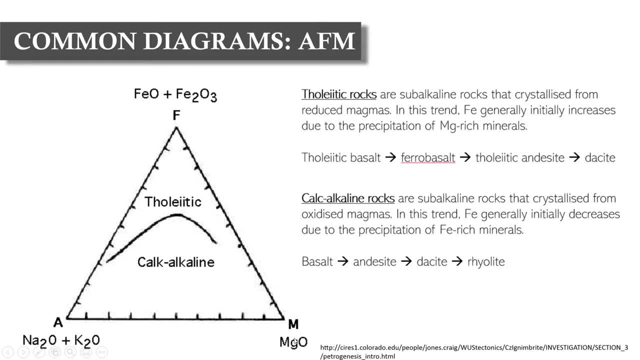 at the top we have our iron, our ferrous and ferric and at the bottom right we have magnesium and in the middle we have sort of this geochemical divide that separates rocks that are considered to be tholeitic and rocks that are considered to be alkaline. Tholeitic rocks are sub-alkaline rocks. 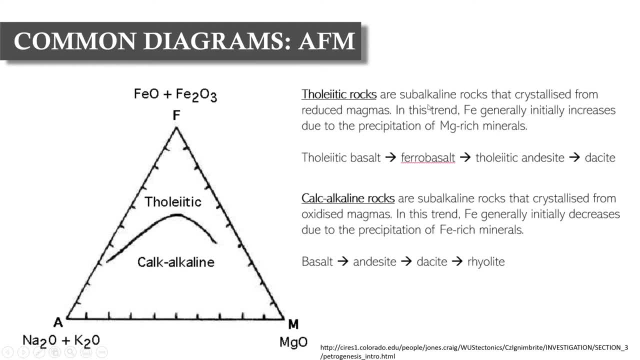 that have crystallized from reduced magmas. In this trend, iron generally initially increases due to the precipitation of magnesium-rich minerals. so as we precipitate minerals such as olivine, the concentration of iron in the magma respectively goes up. In contrast, calc alkaline rocks are sub-alkaline rocks that have crystallized from oxidized 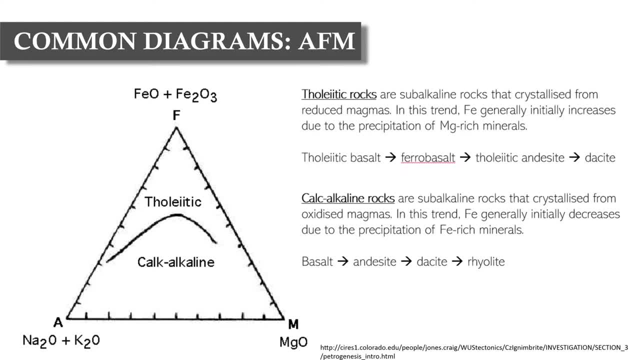 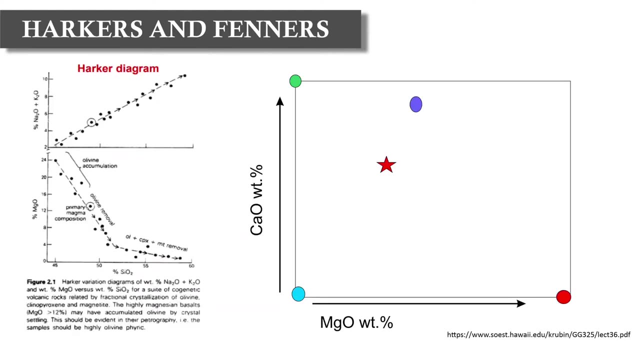 magmas and in this trend, iron concentration initially decreases due to the precipitation of iron-rich minerals. This is quite important about telling us a bit about the oxidation state of our system and also about the geochemical evolution of our system. the liquid line of descents. And that brings us to Harker or Fenner diagrams. Each of these are simple binary diagrams. 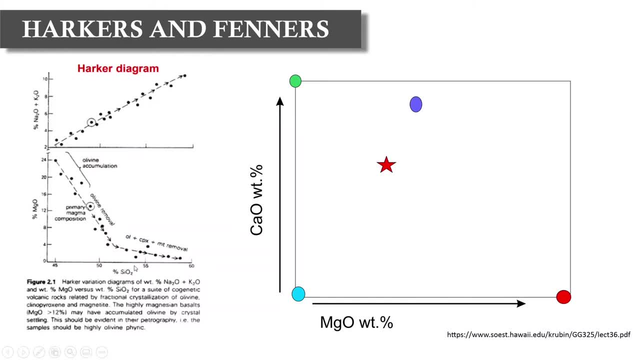 so let's take a look at Harker diagrams to the left hand side. So Harker diagrams are essentially the same as the Harker diagrams to the left hand side. So Harker diagrams are essentially a gauge ay. After these diagrams it can stretch out much further, apart the 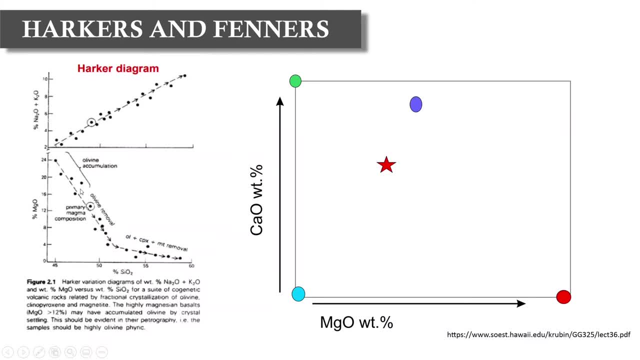 conditions of calc in our lowlands area. However, again we have these two O-g ز, we would say, or in another form, as we said, in thepennings of the thirty three stage form of acidity. so we would feel the same If we had water flows through down the desiccators, two or three. 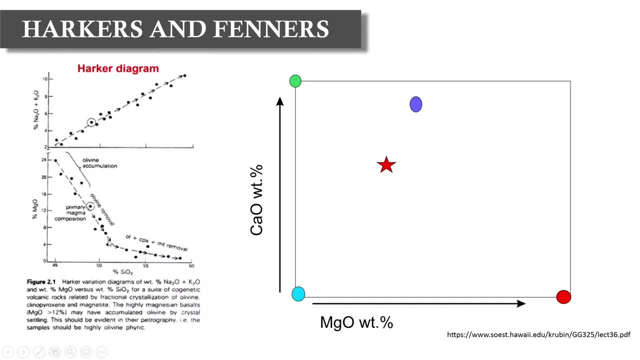 Now we're looking at silica versus magnesium and we can see quite a different trend. And what this is showing us is it's showing us a liquid line of descent, It's showing us the evolution of our rock. So take our primary magma composition here. 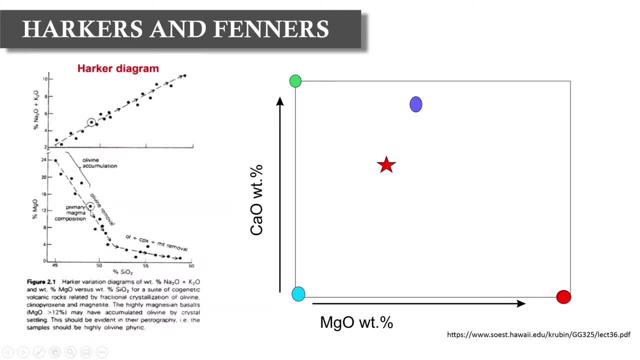 So this is the composition of the magma as it was in place just before. So this is the composition of the magma as it was in place before it started crystallizing Anything more magnesium rich or more silica poor are essentially olivine cumulates. 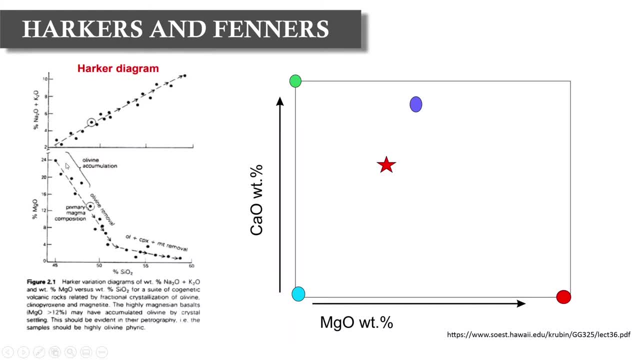 So it's this composition plus cumulates of olivine. OK, so as we add more olivine, obviously the rock gets more rich. in phases that are concentrated in olivine, such as magnesium and concentrations of things like silica, respectively, go down. 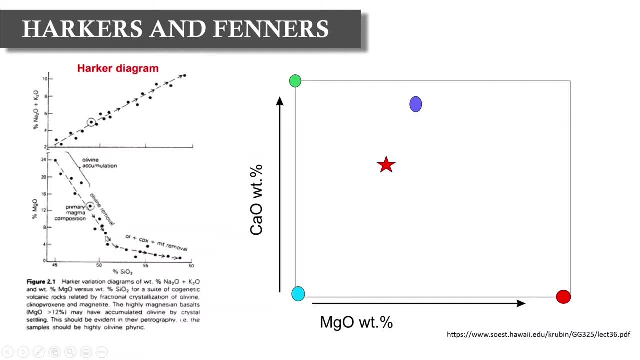 But as we crystallize olivine from this, so we crystallize olivine, olivine, olivine olivine. we remove magnesium from the liquid and we respectively increase it in silica. However, we get to this point and the system changes. 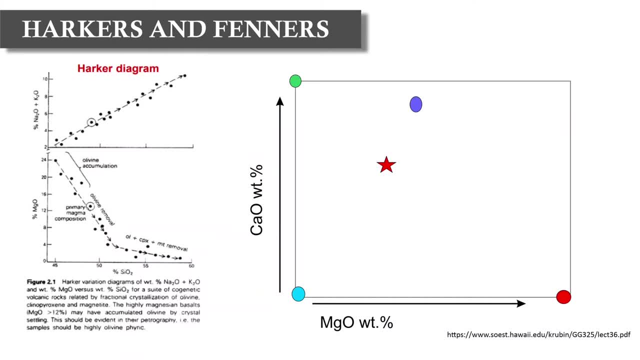 Now we're losing silica a much faster rate than we were before. So now we're no longer just crystallizing olivine, but we're also crystallizing clonoperoxene and magnetite as well. So if we take this example, this is an example of a thinner diagram, which essentially is the same as a Harker diagram, except we have magnesium oxide on the X axis instead of silica. 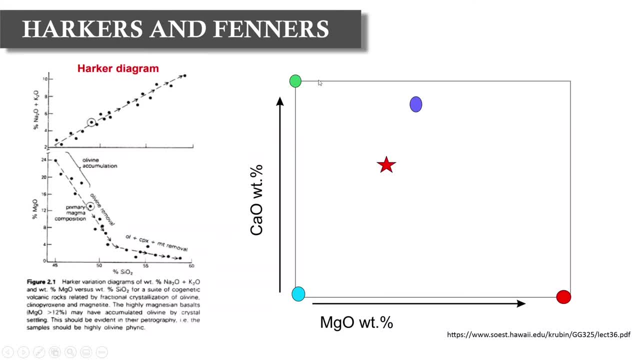 Here is our primary magma composition. This represents pure plagioclase, This represents clonoperoxene, This represents clonoperoxene, This represents quartz or something And this represents olivine. So if we take our primary magma composition, if we just add olivine to this composition, where would a trend of data go? 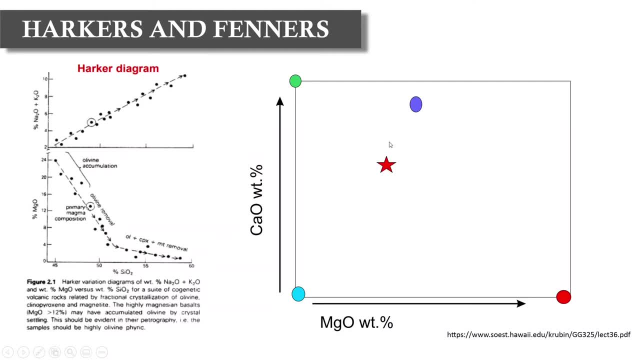 Would it go this way, this way, this way or this way? It would go this way, right? So if we take this composition and we add just olivine to it, that obviously we're going to form a spectrum of rocks that have a variable abundance of olivine. 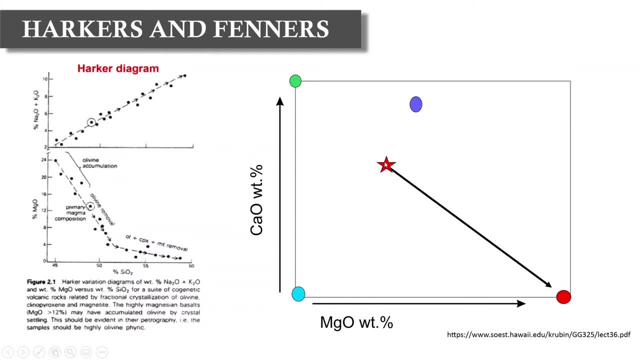 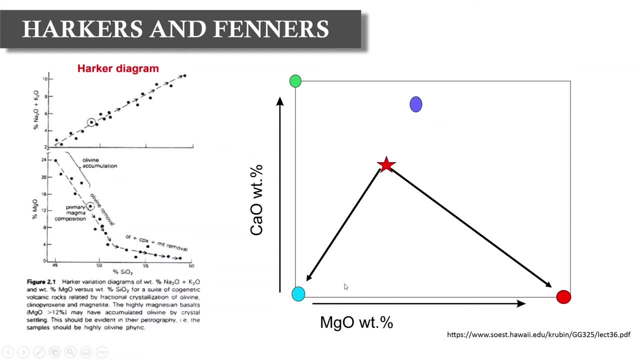 It's going to go this way, right? Because we're crystallizing clonoperoxene, so we're removing magnesium and some degree of calcium, And we're also crystallizing plagioclase, so we're removing calcium, So we're going to be removing calcium at perhaps a slightly faster rate than we're removing magnesium. 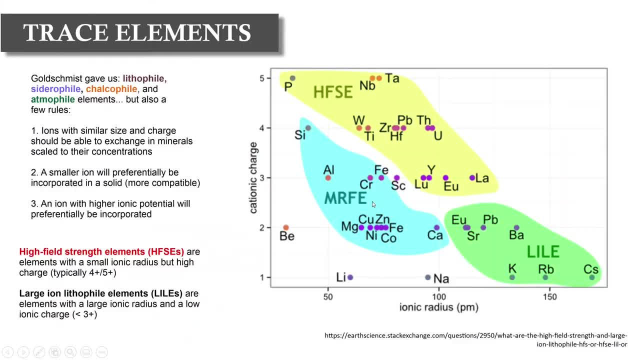 So the rocks are going to evolve this way. So in the igneous petrology series, Goldschmidt gave us lithophile, siderophile, chalcophile and atmophile elements which correspond to rock-loving, iron-loving sulfur or copper-loving, and then vapor-loving elements. 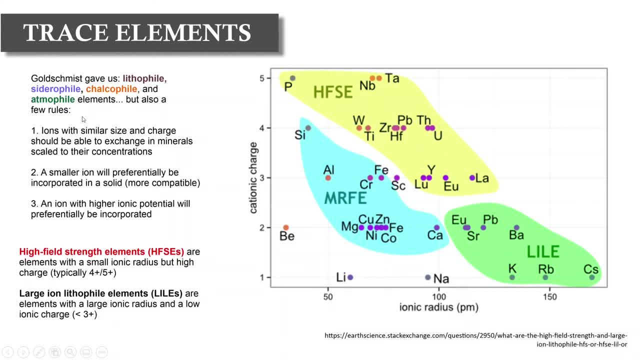 But Goldschmidt also gave us a few rules that tell us a bit more about how a trace element might behave in a geological system. So, firstly, ions of similar size and charge are able to exchange in minerals scaled to their concentrations. So according to the partition coefficient of that element, we may be having substitution reactions happening between a silicate magma. 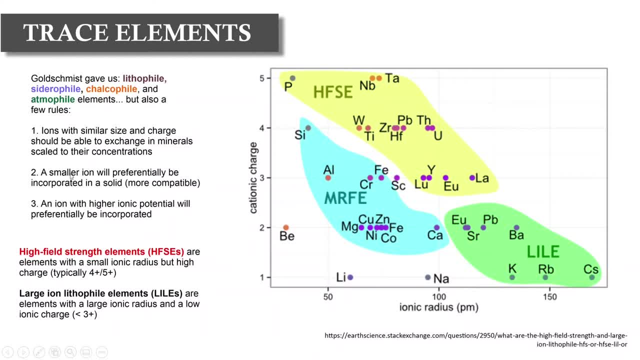 And a mineral phase, and I'll discuss a bit more of that in the next lessons. Second, a smaller ion will preferentially be incorporated into a solid as it's considered. since it's smaller, it'll be slightly more compatible in the crystal lattice. 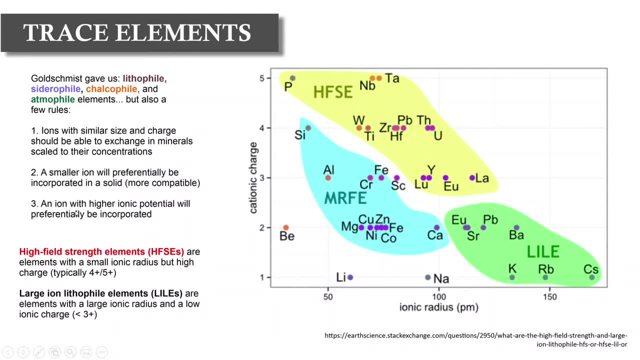 And thirdly, an ion with a higher ionic potential will preferentially be incorporated as, due to its higher potential, is considered to form stronger bonds with the crystal lattice. Now, as always in science, there are exceptions to these rules, but these are a good ways to think about how trace elements might behave. 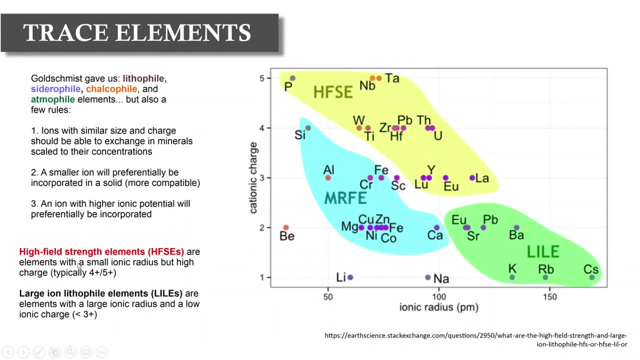 might behave during processes such as crystallisation. And then I get to a couple classifications of what's now considered to be incompatible trace elements. So here this diagram: along the x-axis, we have ionic radius, so the size of our atom, and then we have cationic charge up. 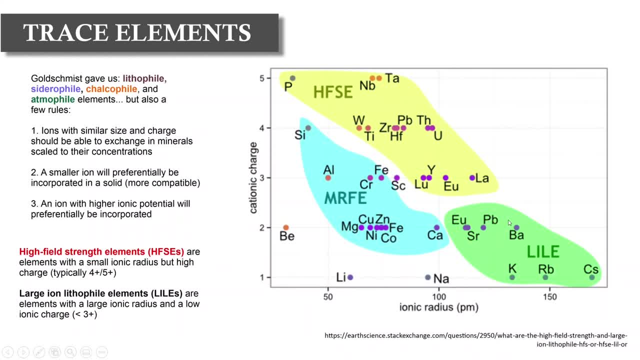 the y-axis, so the valence state of the atom, And I'm most concerned with the green and yellow fields here. So the yellow field is what's referred to as high field strength elements. These are elements that have a small ionic radius but a relatively large valence state. 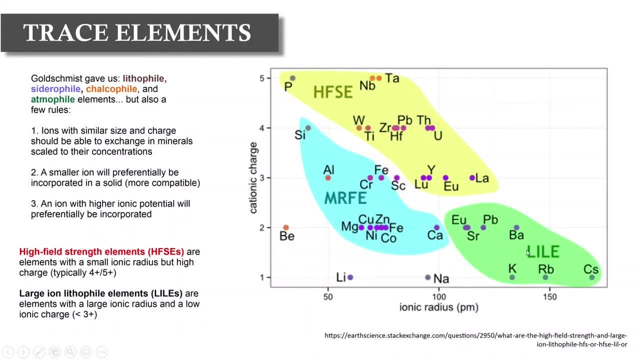 typically above three plus. And then the green fields are LiLe or large ion lithophore elements, and, in contrast to high field strength elements, these have quite a large ionic radius but quite a small cationic charge, And it's through the behaviour of these elements that we can. 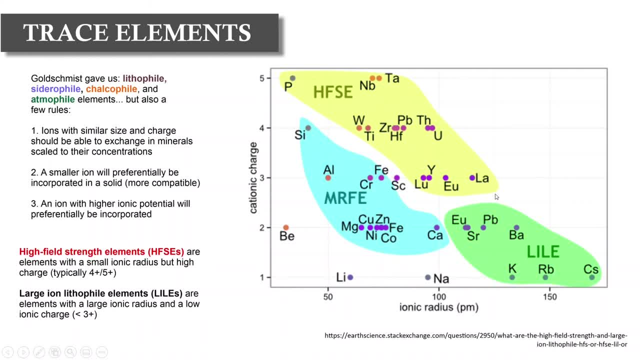 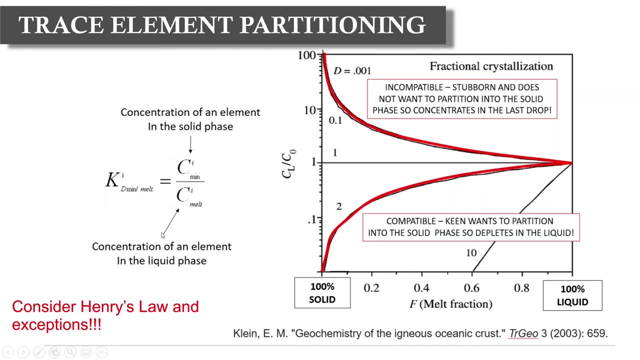 investigate processes such as mantle melting, fractional crystallisation, etc. So trace elements typically behave according to their partition coefficient- and I have a lesson on this in the Ignis Petrology series, if you're like more detail on this- And there are also exceptions to a partition coefficient, and that's. 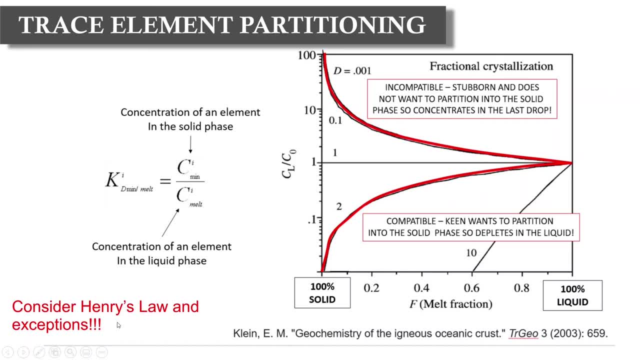 considered in Henry's law, which I do give more detail into in the other lessons, so check that out if you need. So a partition coefficient is essentially a way of quantifying the behaviour of a trace element during geological processes. So what it is is, it is a concentration of a phase. 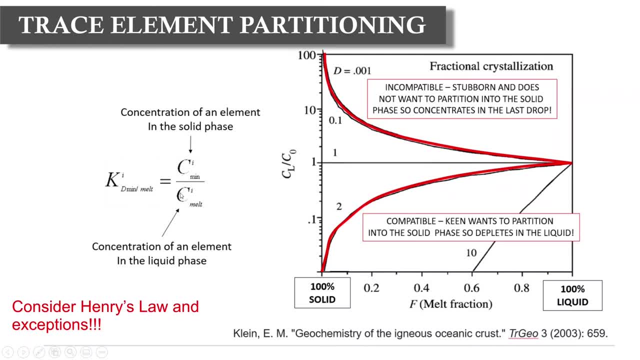 in a mineral and then the concentration of that phase in a corresponding silicate melt. And it's through undergoing this reaction we look at the degree of enrichment or depletion of that element in a mineral phase relative to the silicate melt. So let's take this diagram as an example. 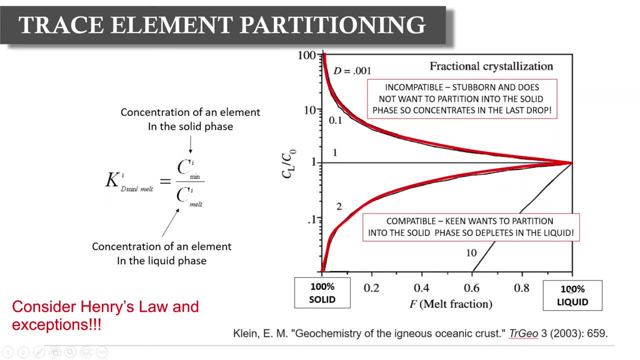 So on the x-axis we have the concentration of liquid. so over here we have 100% liquid, over here we have 100% solid, ie 100% crystalline, and in the middle we have a mixture of liquid and solid. At the y-axis we have the concentration of the element in the liquid. 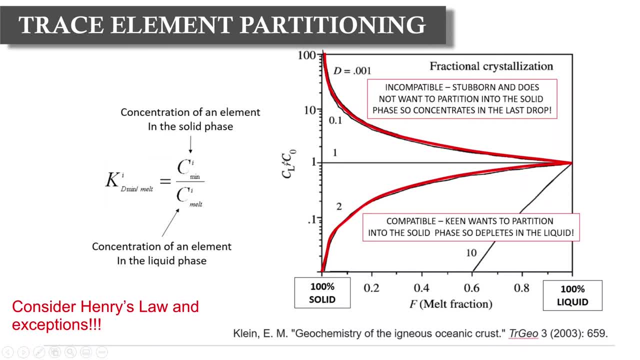 and concentration of the element in the solid. So, because it's concentration in the liquid, as we go up here the element is more enriched in the liquid relative to the solid, and as we go down here, the element is more enriched in the solid relative to the liquid. And all these numbers in here. 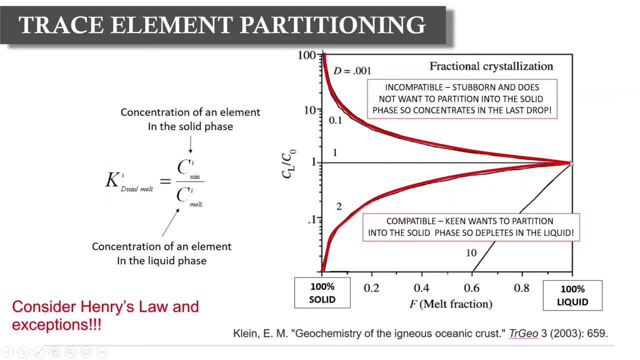 correspond to different partition coefficients. So say, we start here and we're going to look at the behaviour of an element with a partition coefficient of 2, so ie slightly compatible. What it's going to do is, as the liquid crystallises a solid phase, this element is 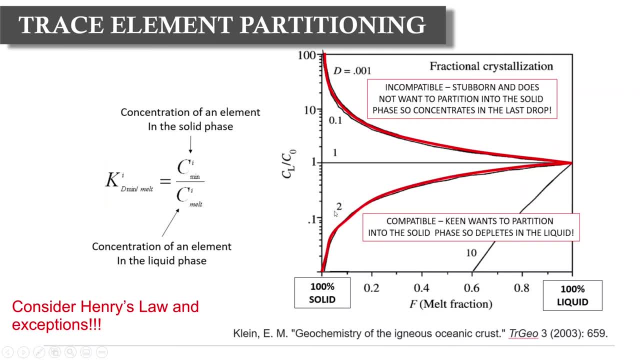 going to preferentially be removed due to its higher compatibility, due to its higher partition coefficient. So as there's more solid, more solid, more solid, this element is preferentially removed. Conversely, if we have an incompatible element which is slightly stubborn and it wants to stay,